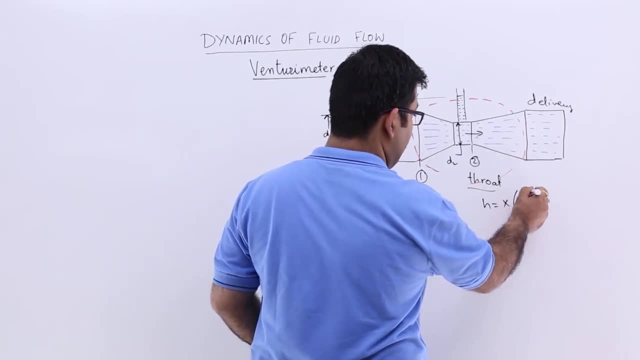 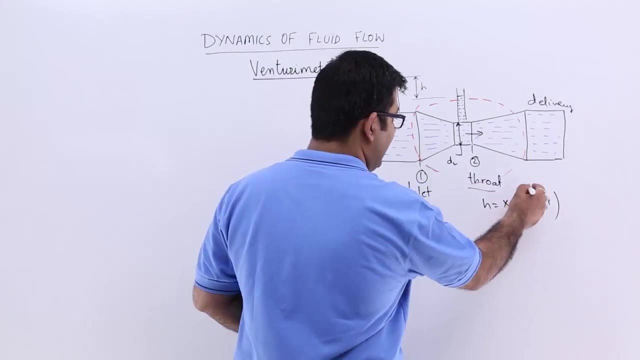 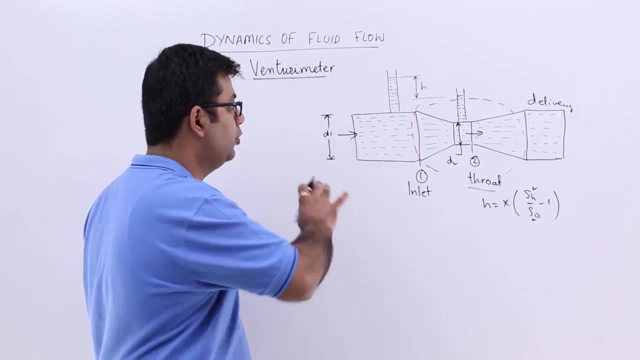 manometer i can use. h is equal to x into sh upon s, not minus one, where x is the reading of the manometer and sh is the specific gravity of the heavier liquid and s not, is the specific gravity of the liquid which is flowing inside this pipe. okay, so this is how you can find. 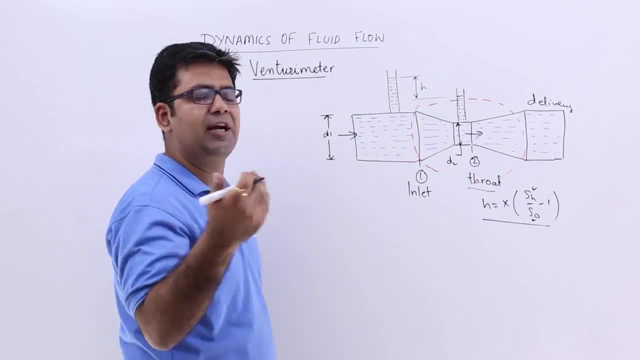 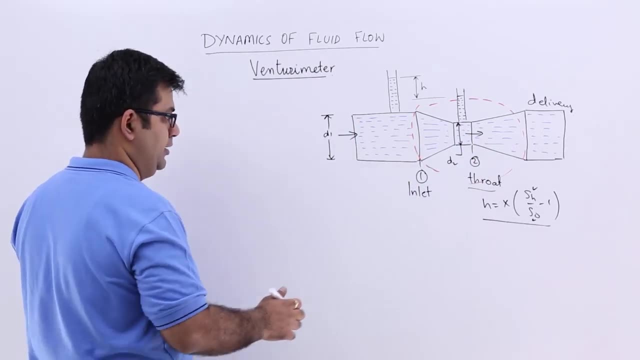 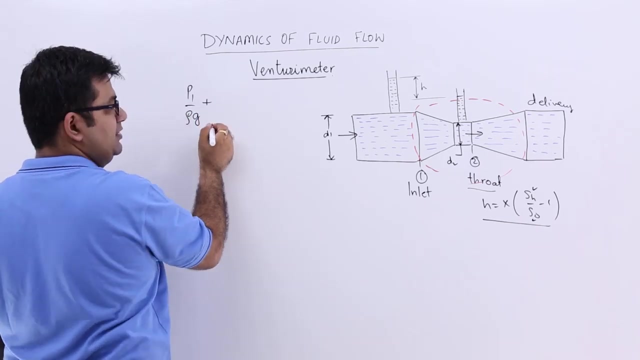 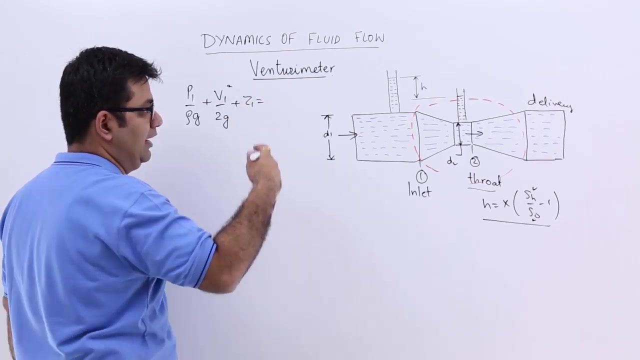 out h. now let's start applying the bernoulli's equation in between these two sections. alright, so let's apply on section one, so you will have. let's write down here, so you will have: p1 upon rho, g plus v1 upon 2g plus z1 is equal to, so that will be the total energy. 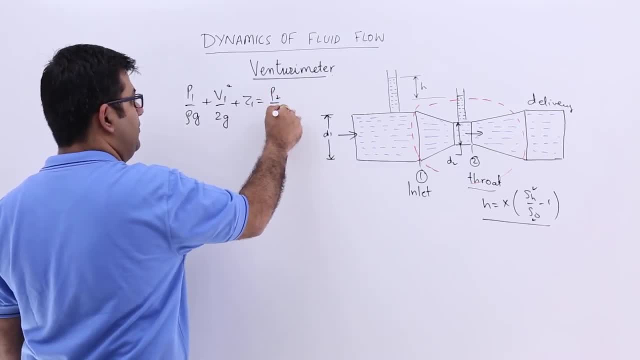 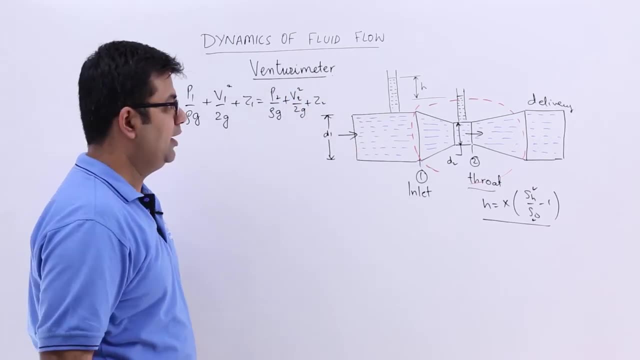 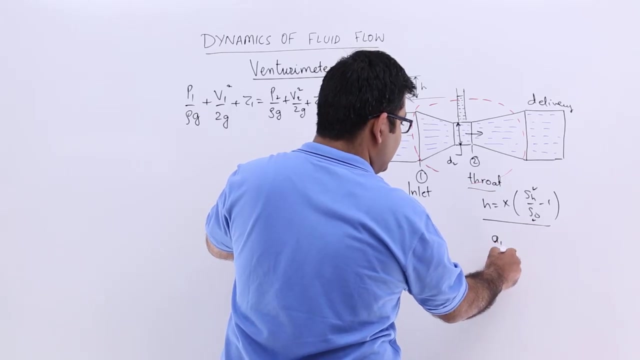 on the section two. so it will be equal to p2 upon rho. g plus v2, square upon 2g plus z2. okay Now, Because you have got the diameters at d1 and d2, you can find out the areas at these two. 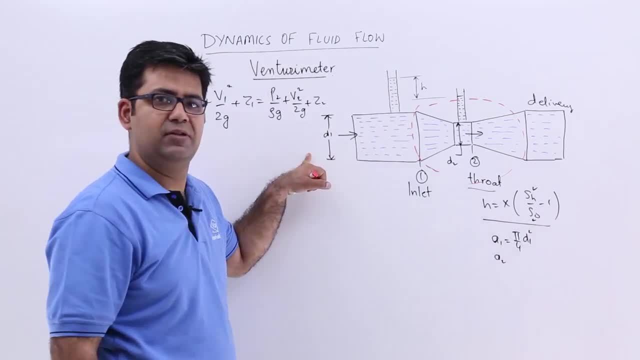 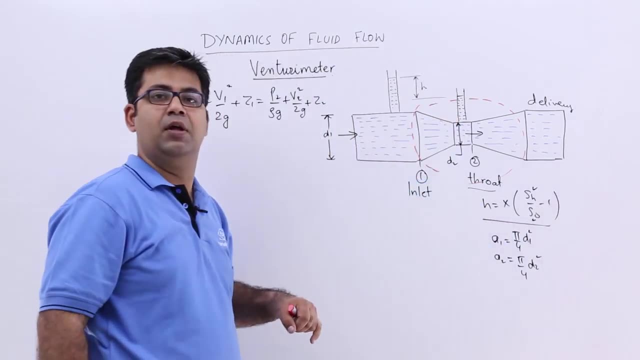 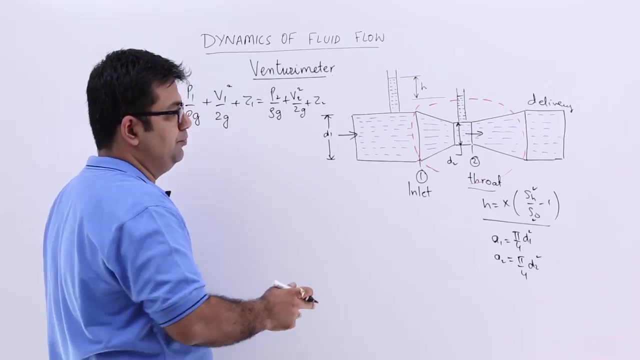 sections. so a1 would be pi by 4 d1 square and a2 would be pi by 4 d2 square. alright, now we will use that at some place. so right now i can say that for both these sections i can assume this as the datum. 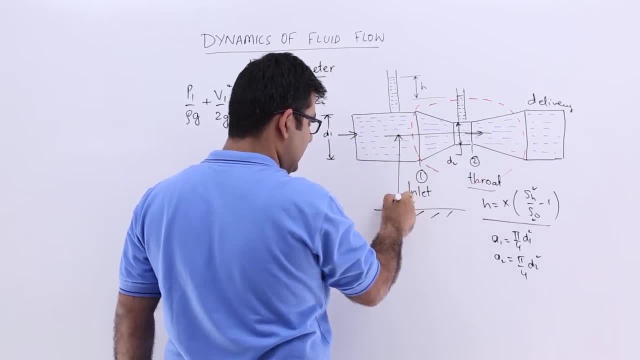 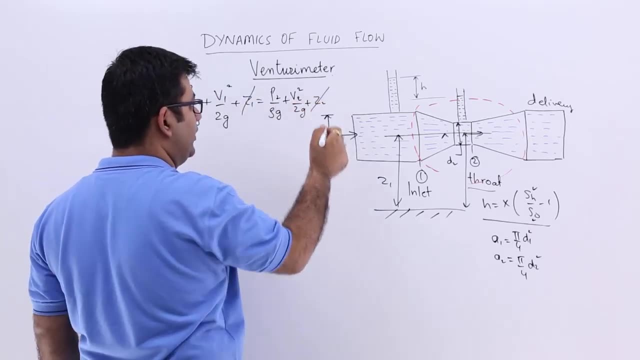 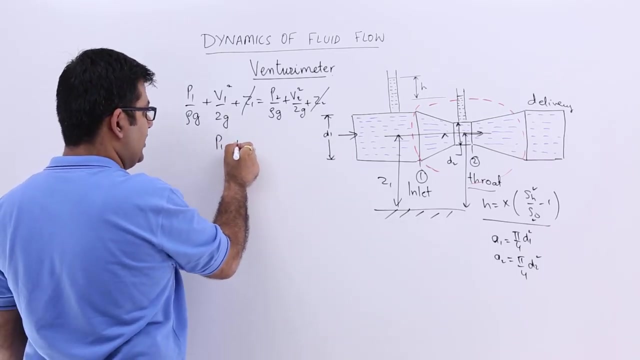 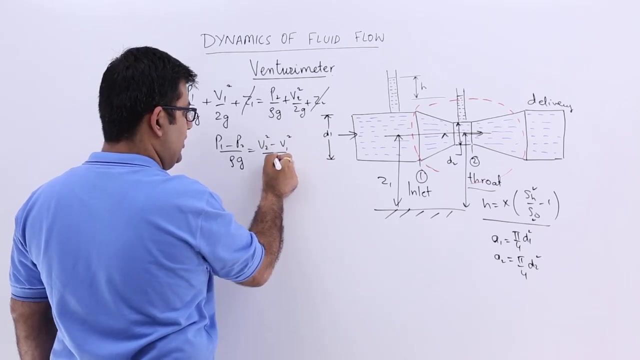 So Let us say this is the section height, z1, and then this would be z2, so the height is same. so i can strike off z1 and z2. alright, so now let me bring p2 over here and v1 over there, so you will get p1 minus p2 upon rho. g is equal to v2 square minus v1 square upon 2g. 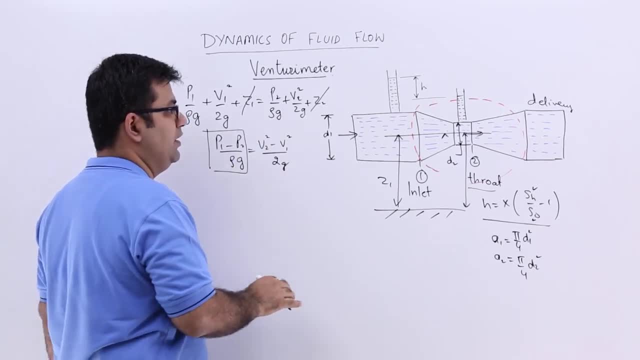 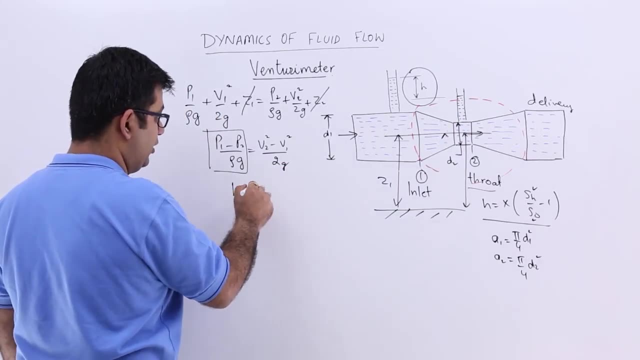 let us say this is the pressure head difference between sections, So So, So This is section 1 and section 2 in that is represented by this height, h. so this is h. you can also calculate h with this formula, okay, so h is represented by this, which is: 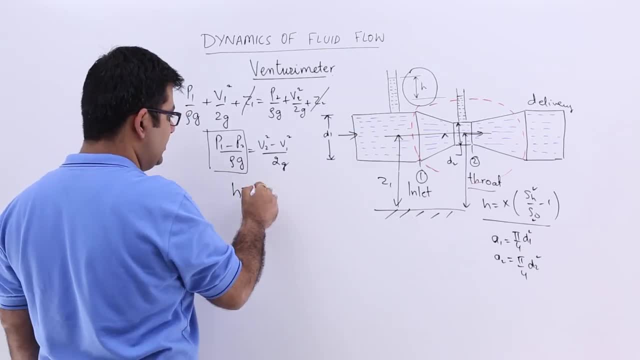 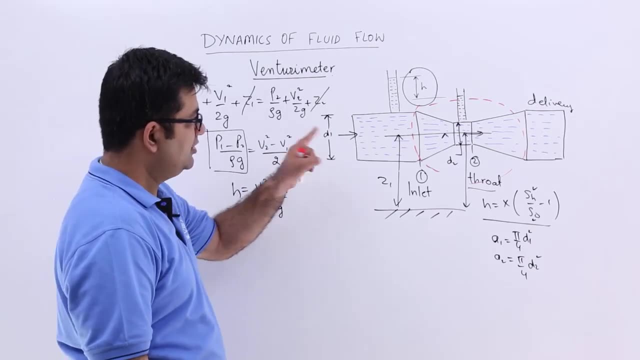 the pressure head difference at the two sections, and this is v2 square minus v1 square upon 2g. now, because of the continuity, equation is applicable over here, so i can say that a1- d1 is equal to at 2.. Now So, 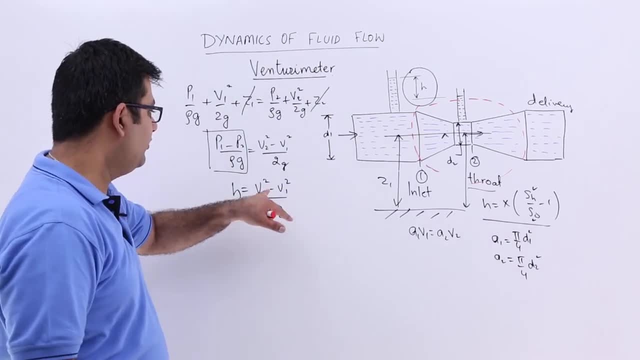 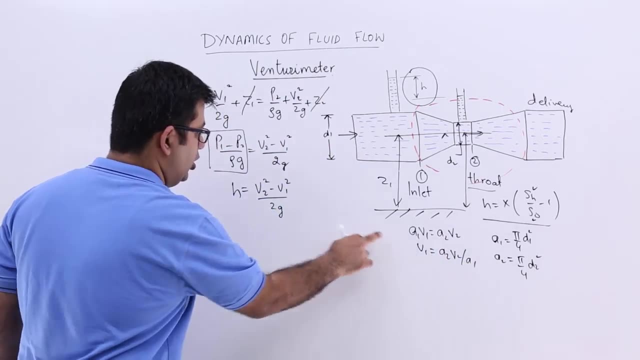 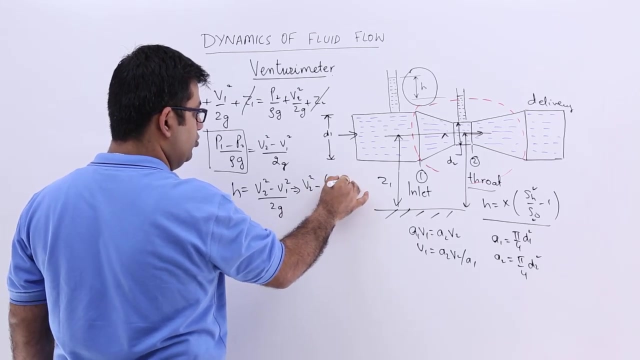 a2, v2.. Let's find out the value for v1.. So v1 would be a2 into v2 upon a1.. Let's substitute this over here, So I will get v2 square minus a2 into v2 upon v1, whole square upon this. 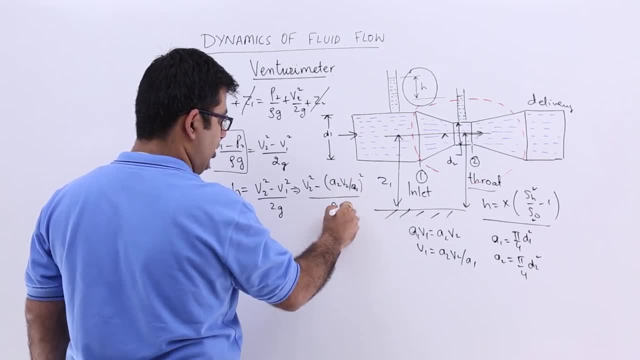 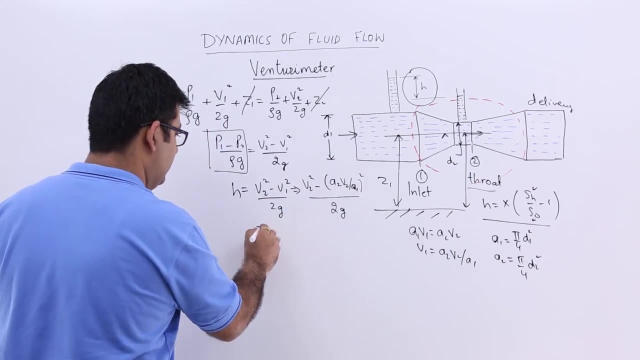 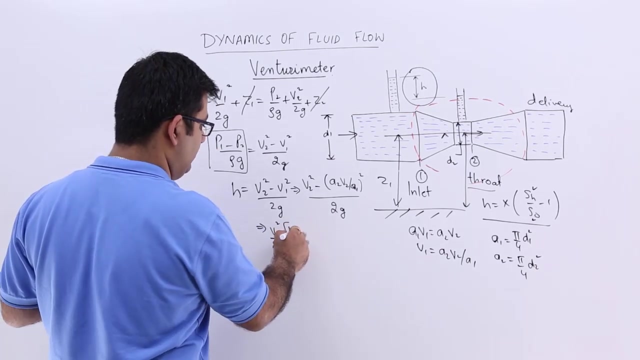 is a1 whole square upon 2g. I can take out v2 square upon 2g common, So I will have v2 square upon 2g as a common value and then in the bracket I will have 1 minus a2 upon. 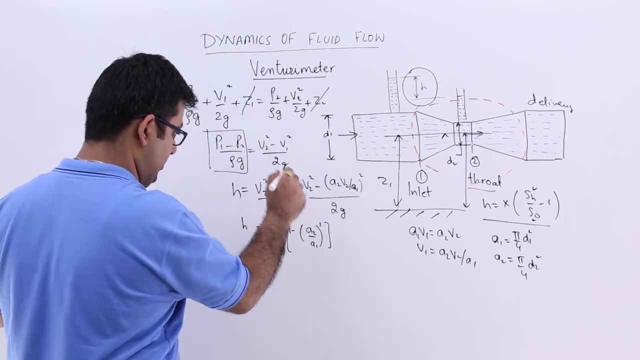 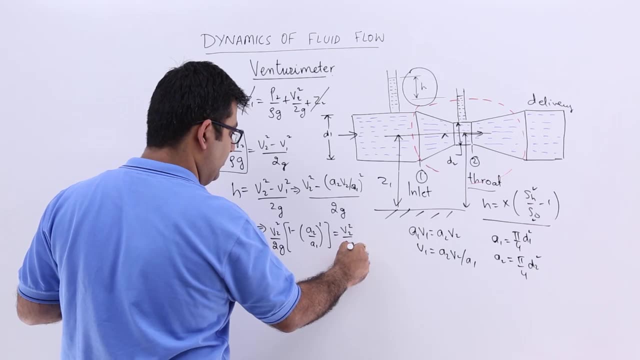 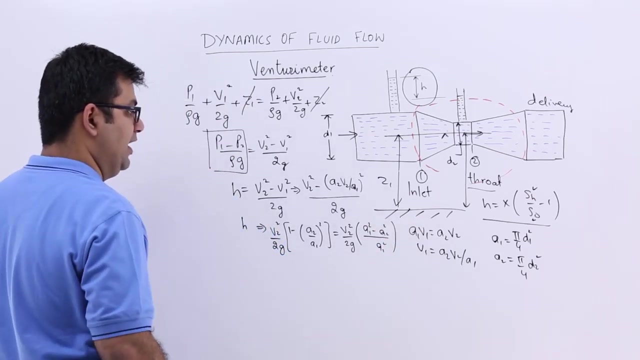 a1 whole square and this is h. Okay, and further simplifying this, I would get v2 square upon 2g. So I will take out 2g into a1 square minus a2 square upon a1 square, and from here we are more interested to find out the value for v2, because we already know a2.. If we get 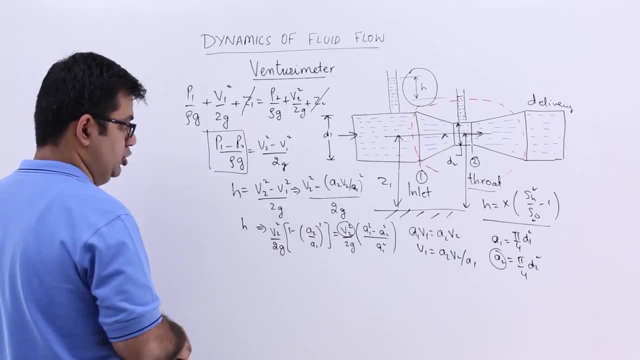 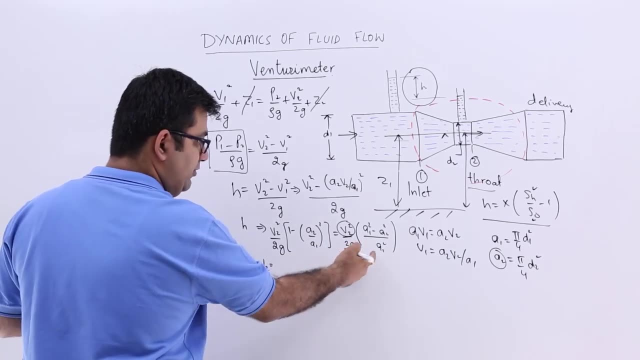 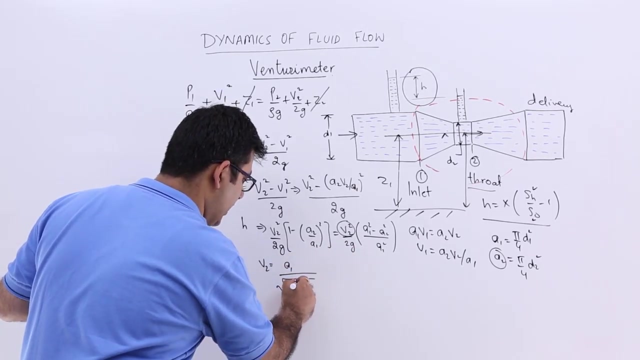 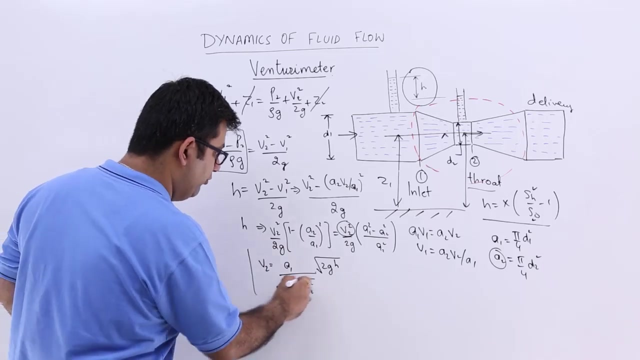 the value for v2, we can easily find out the discharge. So from here, v2 would be under root 2gh and this will become only a1 because it is a single value upon under root 2gh. So that is the value for v2.. If I have to find out the discharge through this, Venturi. 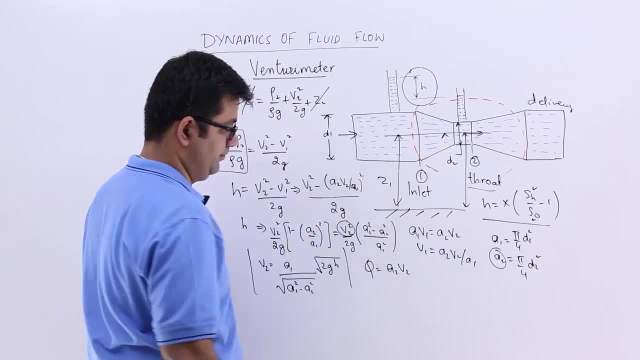 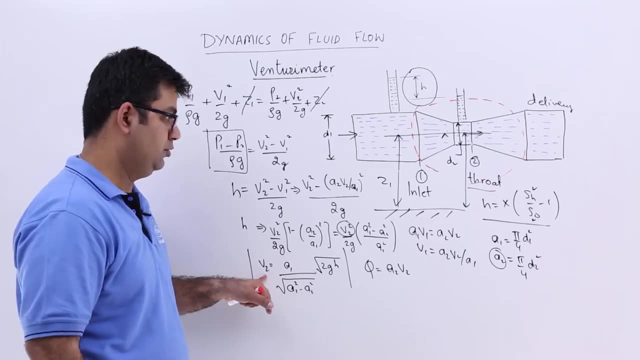 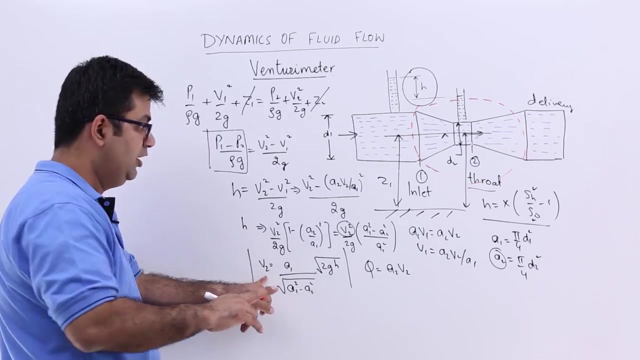 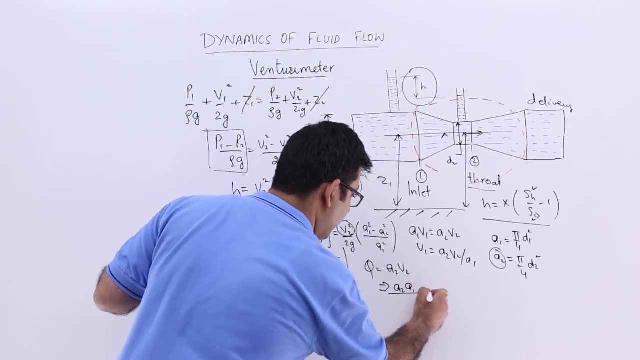 so q is equal to a2- into v2. you can also substitute for v2 over here, So you will get the value for v1.. Okay, so no need to go by only this method. You can also substitute for v2.. Now we have found out the value for V2, so let us use that. so you will get A2 into A1 upon.